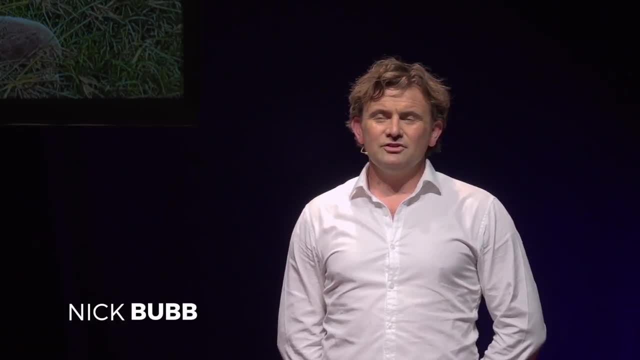 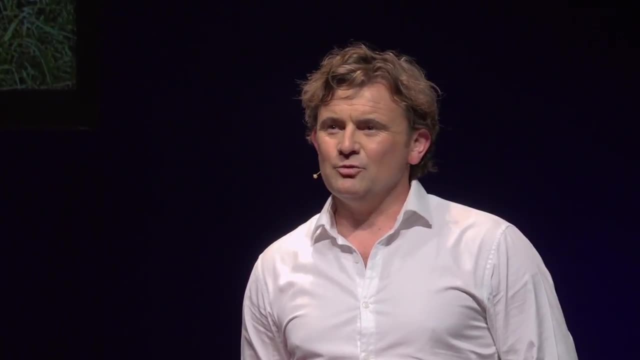 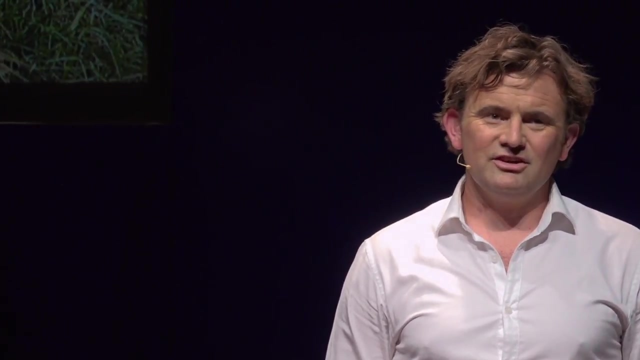 become used to humans. This afternoon, I want to remind you all about the value of nature. I want to tell you what we can all do to help protect the natural world and why working in wildlife conservation is one of the most exciting, dynamic, interesting and rewarding. 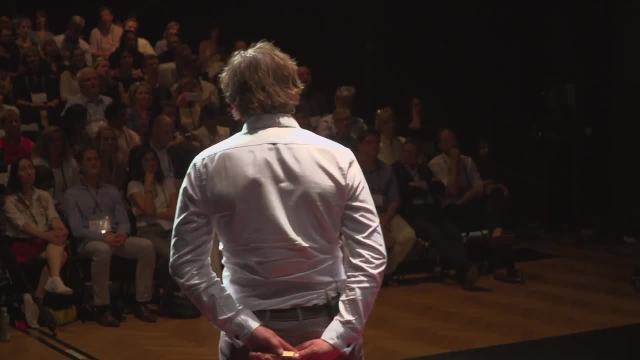 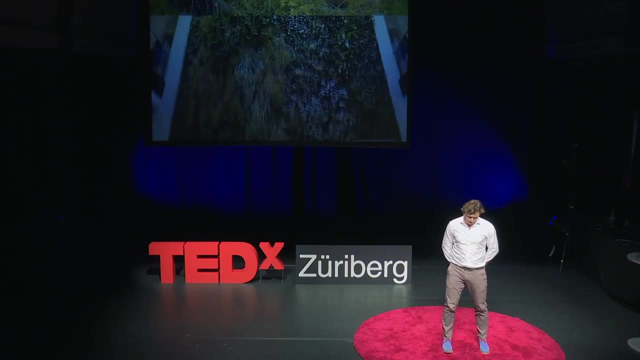 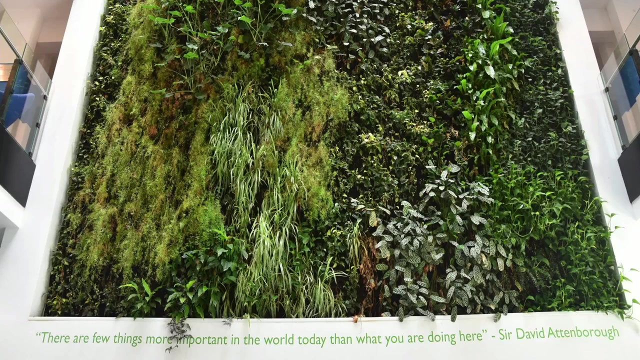 roles you can ever have. The idea that I want to share with you all is that there is a role for everyone in wildlife conservation. There are a few things more important in the world today than what you are doing here. These inspirational words from Sir David Attenborough: 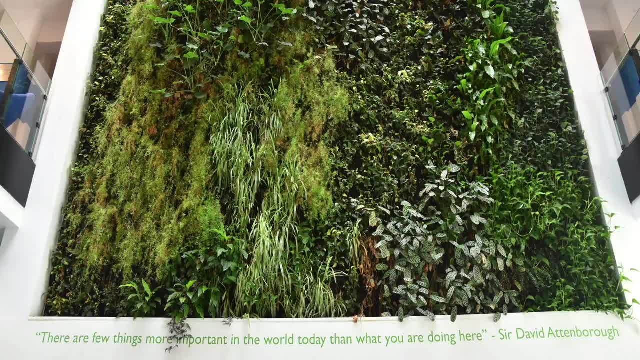 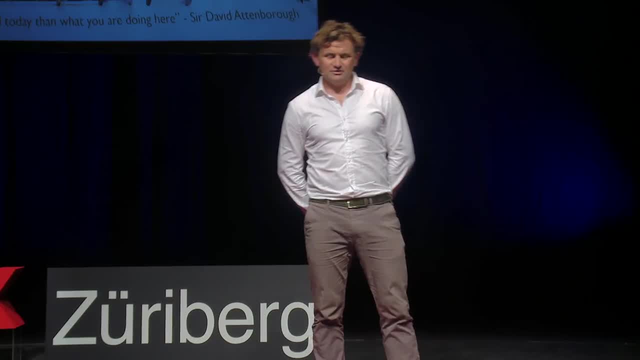 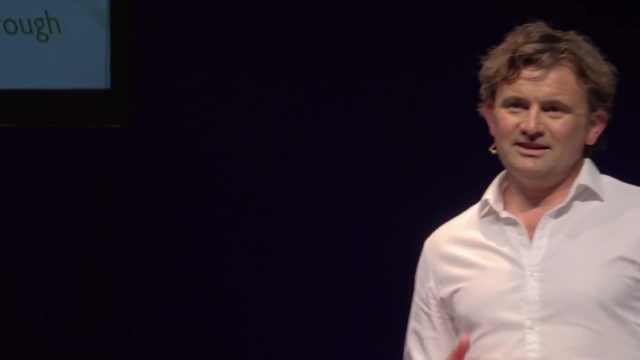 are written on the living wall when you enter the Sir David Attenborough building, which is home to the Cambridge Conservation Initiative and 10 of the world's leading biodiversity conservation organisations. It always inspires me when I walk through those doors and leaves me excited, and it's that excitement that I'd like to share with you all today, and 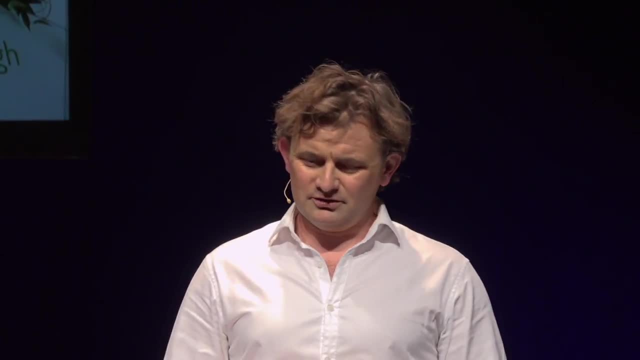 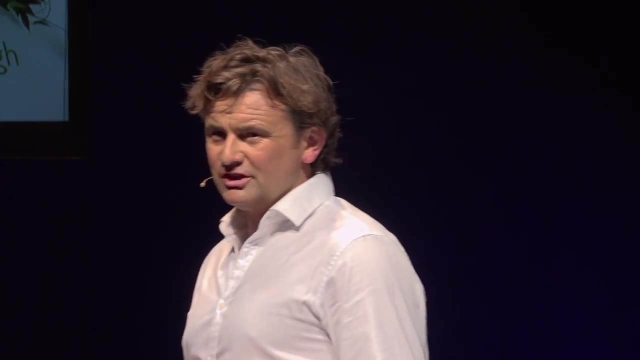 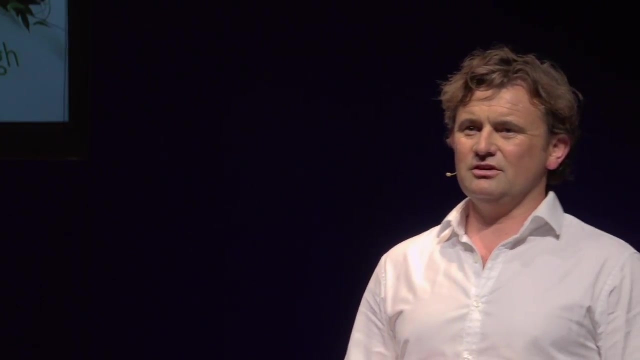 I hope that you all leave here empowered to help protect the natural world too. To kick off, I want to demonstrate the value of nature: Agriculture, tourism, fishing- fishing which, by the way, is worth 300 billion US dollars to global GDP. 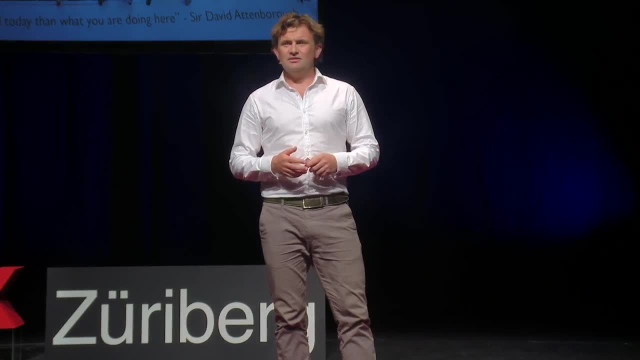 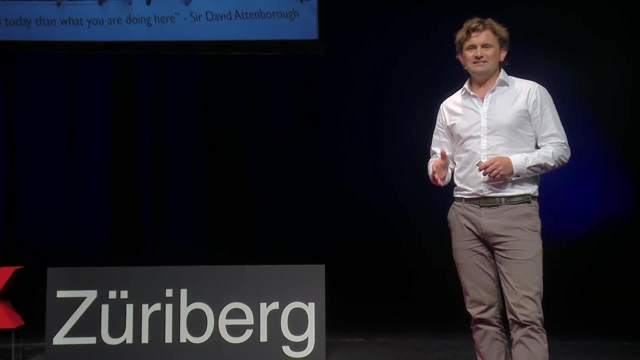 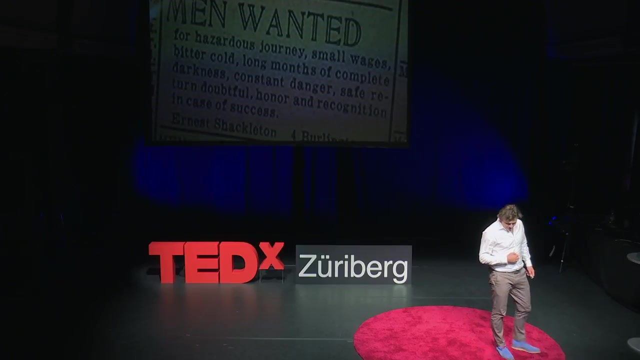 Medicine, energy, clean water- they're all examples of nature sustaining our economy and our welfare. Nature is the very basis of our welfare and economy, and it's critical that we manage it correctly. Men wanted for hazardous journeys, small wages, bitter cold. 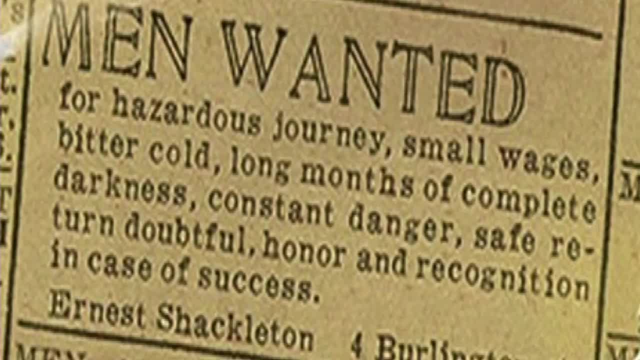 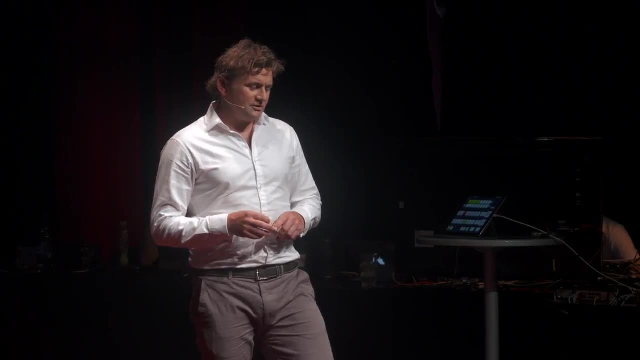 long months of complete darkness, constant danger, safe return, doubtful honour and recognition in case of success. Sometimes I think I'm describing my current job, but this is an advert that some of you might recognise that Sir Ernest Shackleton placed in the Times in 1914.. What was to follow was one of the greatest survival stories of all. 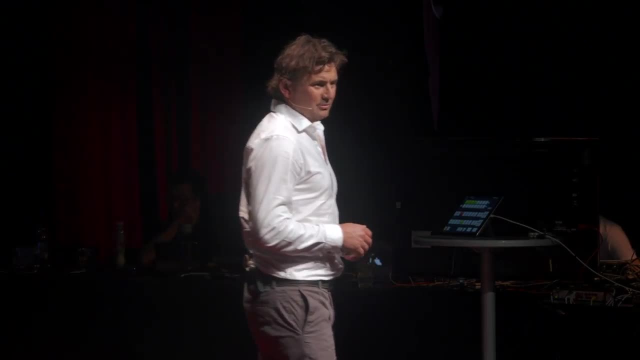 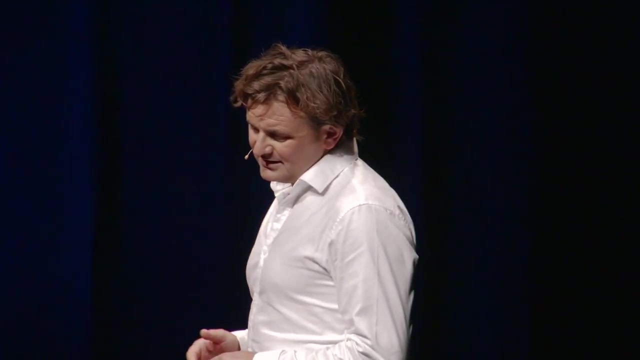 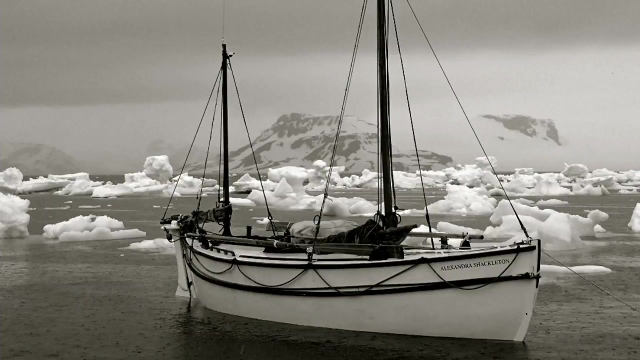 time and an example of inspirational leadership in adversity. So how does this connect to conservation? Well, five or nearly six years ago now, I was invited to skip a project, an expedition that was part of a Discovery Channel documentary that was going to retrace Sir Ernest Shackleton's voyage. 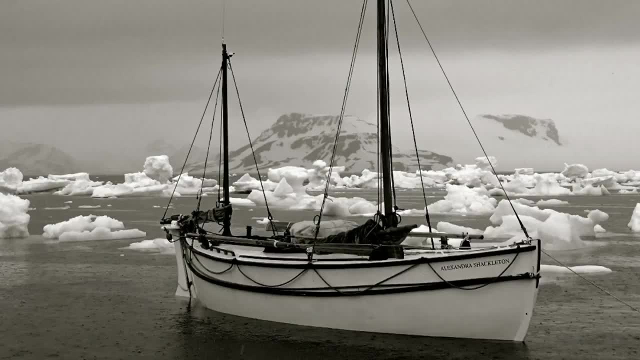 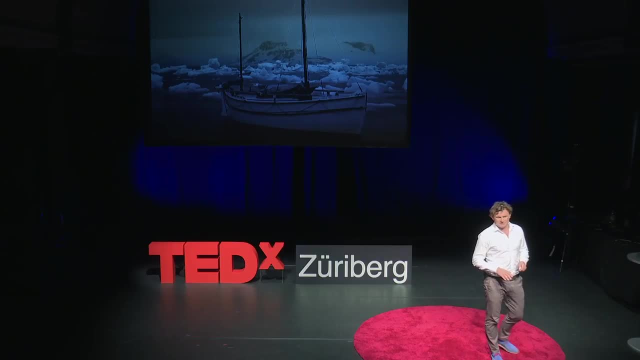 One hundred years after it first occurred. we were going to use a replica boat, such as the one you see here, and replica kit. What we were also going to do was document climate change in the intervening years. It was simple stuff. It was what I would call. 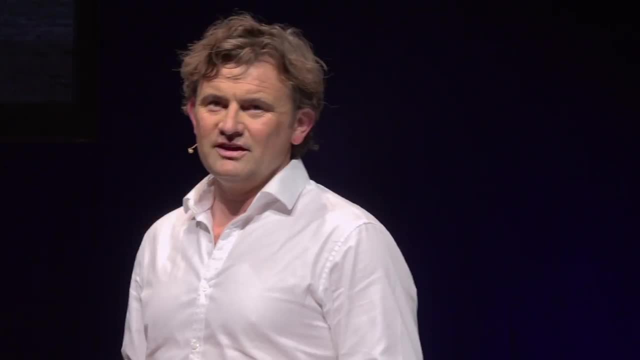 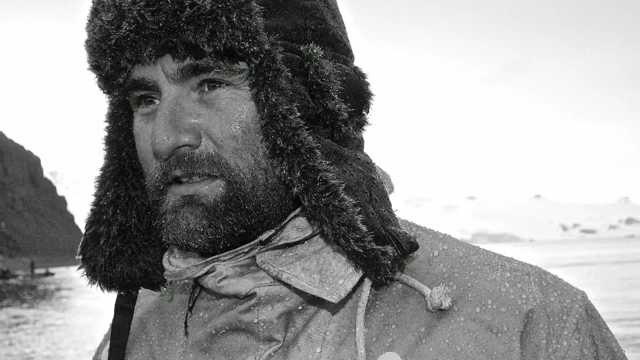 citizen science, So looking, for instance, at how far the glaciers had retreated during that time. For those of you wondering, this is me how I might have looked a hundred years ago. Stepping back in time, though, and seeing first. 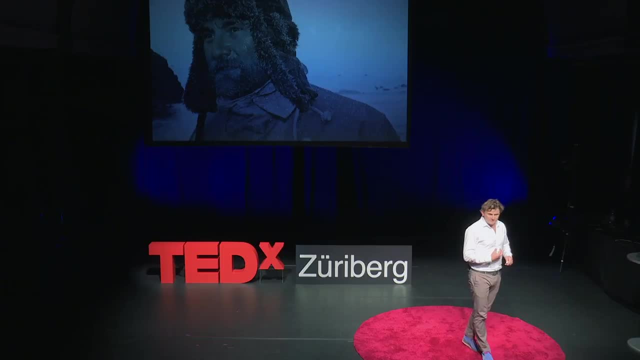 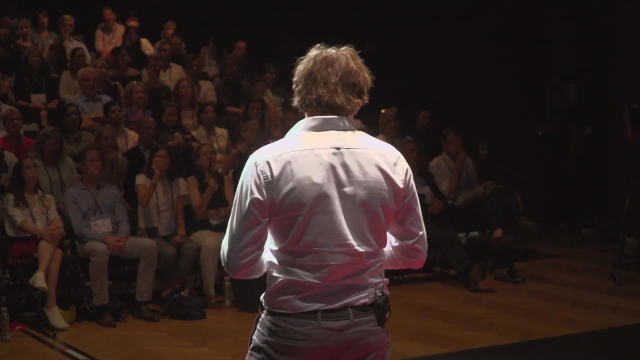 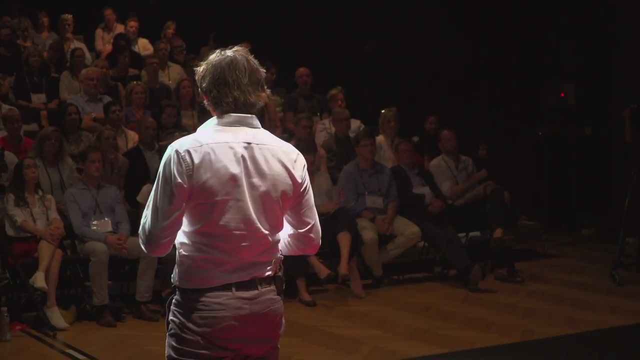 hand, the impact of climate change really changed me too, And during the expedition we raised funds for an organisation called Fauna and Flora International FFI, a biodiversity conservation organisation protecting critically endangered species and habitats. And, to cut a long story short, I came back to the UK and had a lot of conversations with the CEO. 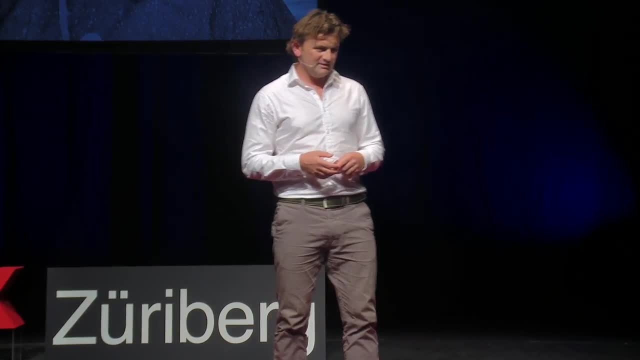 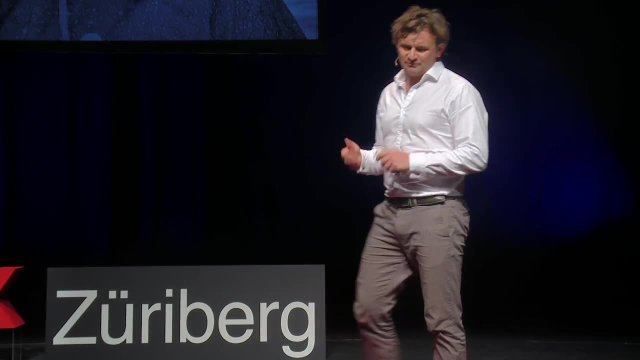 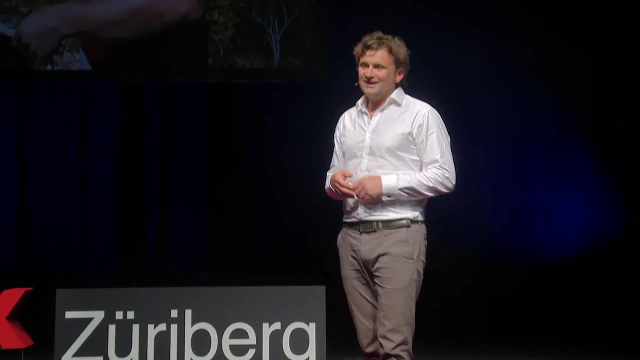 bothered him for a long time and eventually he offered me a role promoting the organisation, and the organisation has been in existence for a hundred and fifteen years. The role that I have is mainly in a suit working the boardrooms and conferences forums. 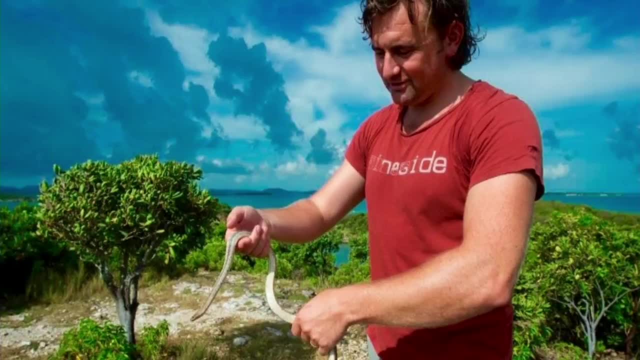 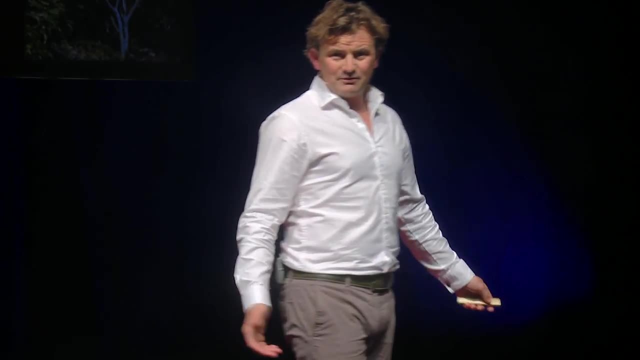 but sometimes I get out in the field, and here I'm tagging a critically endangered Antiguan racer snake. I also get to visit some of the most amazing projects all over the world, And I've been with FFI now for five years, but my background is actually I'm an engineer. I've worked in finance and probably, or in fact, I've been in the industry for a long time. I've been in the industry for a long time and I've been in the industry for a long time. and I've been in the industry for a long time and I've been in the industry for. 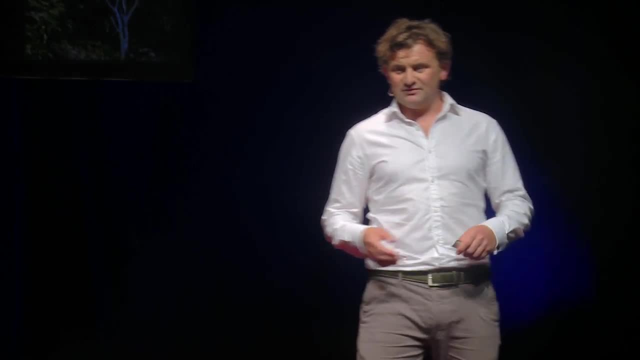 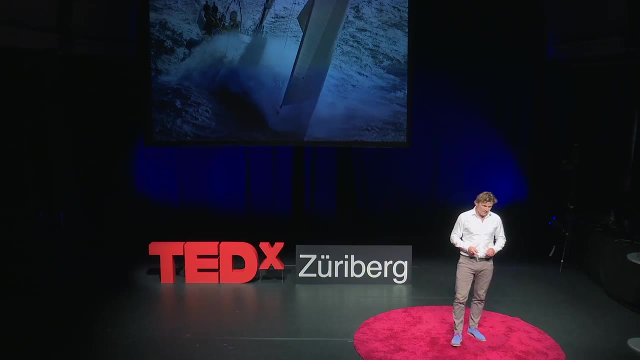 a long time, In fact, definitely. more interestingly, I was also a professional offshore sailor for ten years, competing in events such as the Volvo Ocean Race in 2008.. So I've had a wide range in career, but I am definitely no zoologist. I didn't grow. 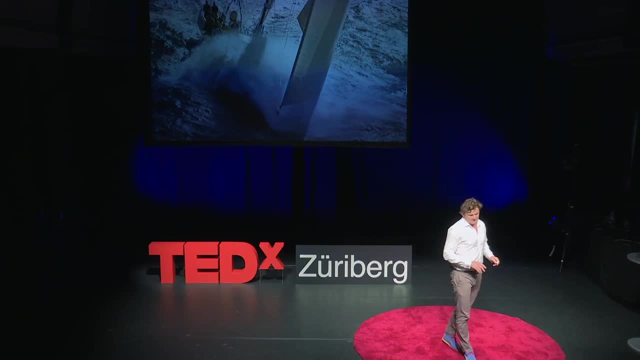 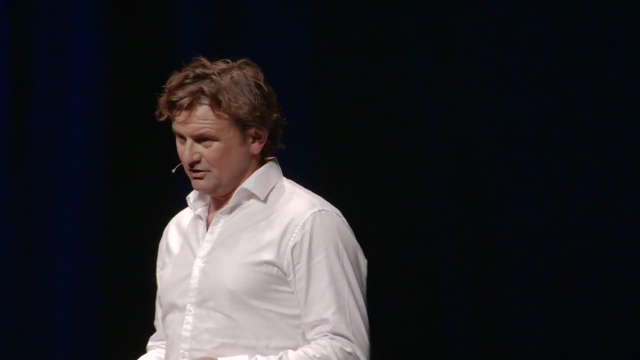 up in Africa. I don't know the Latin names of any plants and well, I suppose what I am is I'm a passionate advocate for the importance of protecting the natural world, And there are actually lots of conservationisng in nature. I don't know if you know this. I 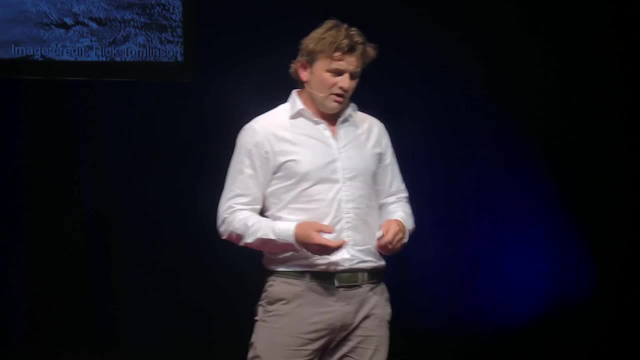 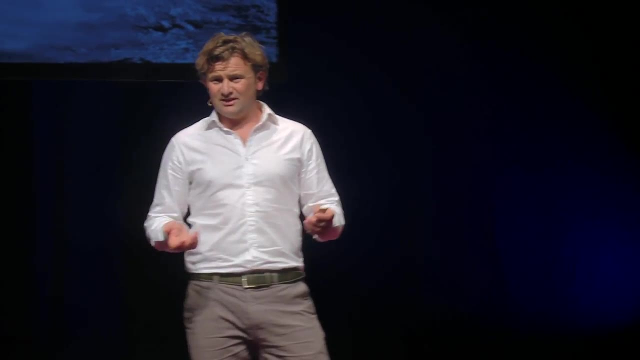 often raise fale on the bottom ofEE conservationists like me that come without formal training. Of course, many of us- in fact most of us, are zoologists, ecologists, naturalists, primatologists and, fundamentally, scientists. And, yes, many of my colleagues grew up keeping pet worms and collecting snail. 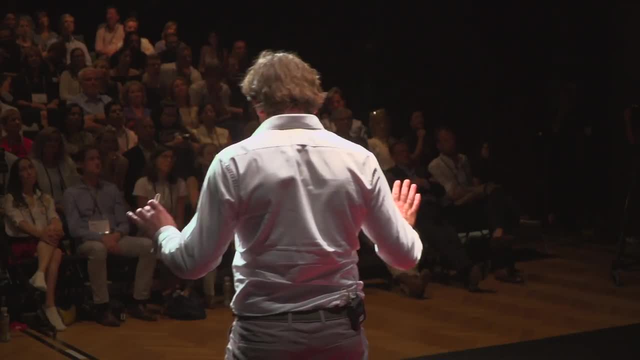 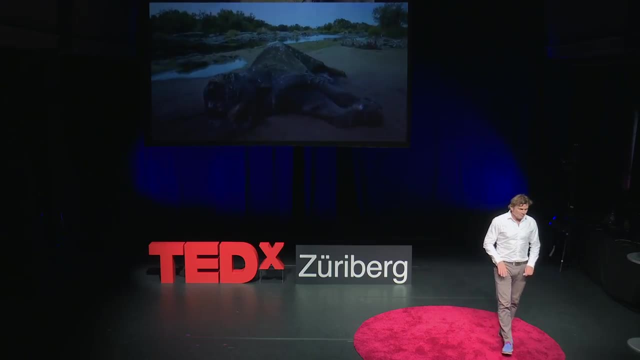 shells And, yes, many of them love hugging trees, But hey, nowadays even I enjoy doing that with my son, Even if I am a paper conservationist. I'll come back to that, But before we get too comfortable, I think we all need a dose of reality. In 2013,, 20,000 wild elephants. 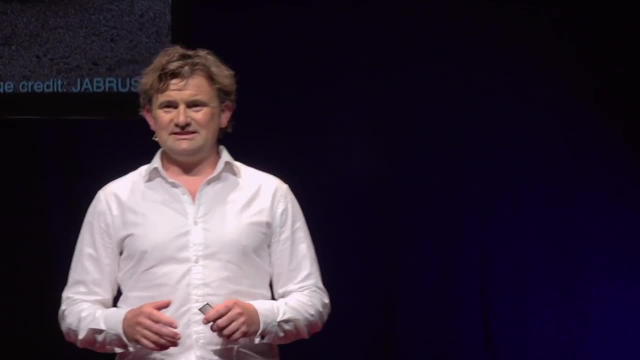 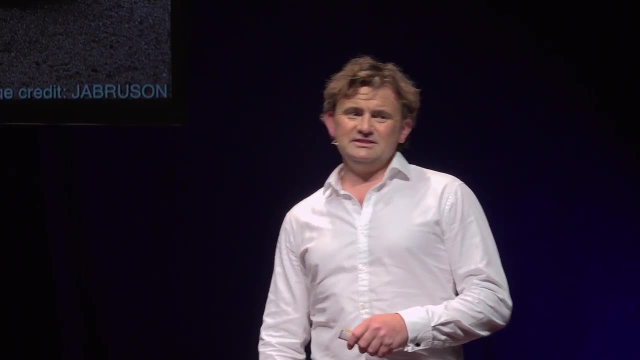 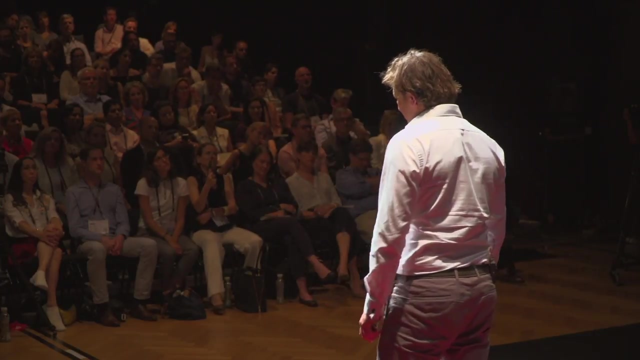 were killed. The lion population is down 40% in the past 20 years and there are only 3,000 tigers left in the wild. This iconic species could become extinct within our lifetime. In the last 10 years, 7,500 African rhinos have been poached. 1,000 rhino were poached. 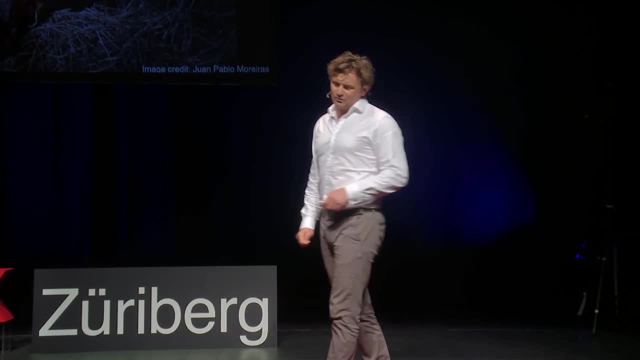 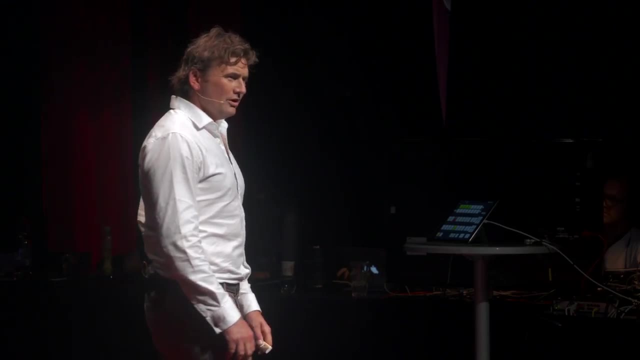 in 2017.. In 2010,, the western black rhino sadly became extinct and the last male northern white rhino died in March. Why all this slaughter? Well, rhino ivory is now worth in excess of 60,000 US. 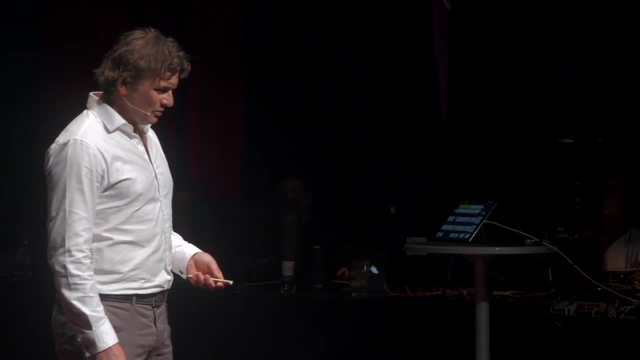 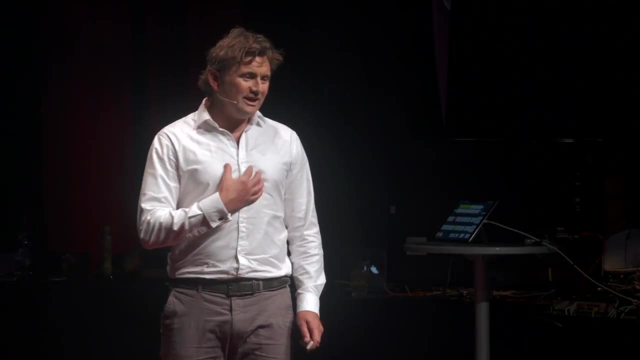 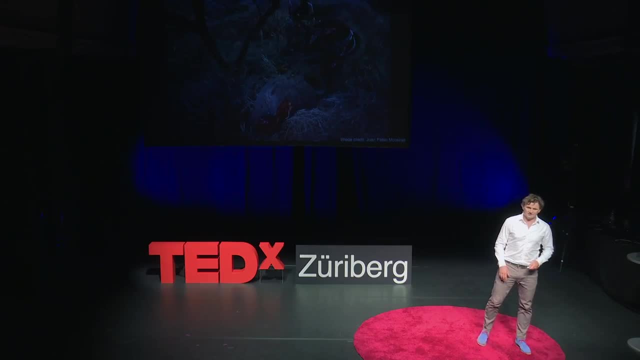 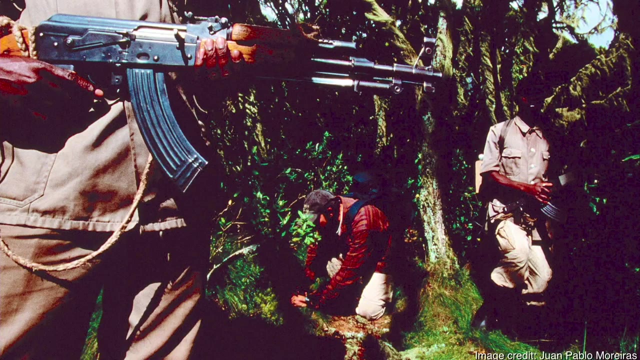 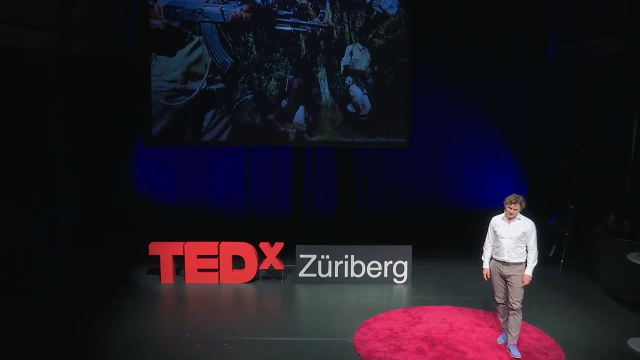 tracking and in protecting these wildlife, to work alongside our rangers and our scouts, No more so than in the Virunga National Park, which spans DRC, Rwanda and Uganda and is home to the critically endangered and iconic mountain gorillas, But it's also home to militia. 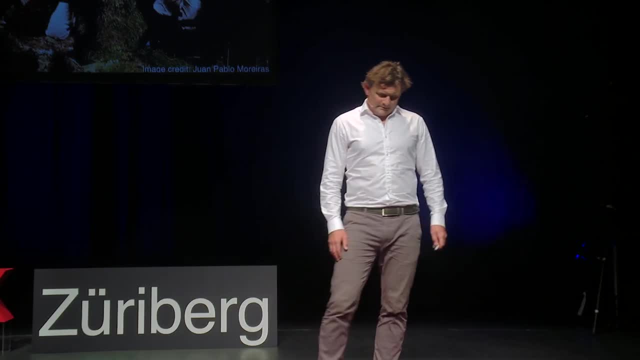 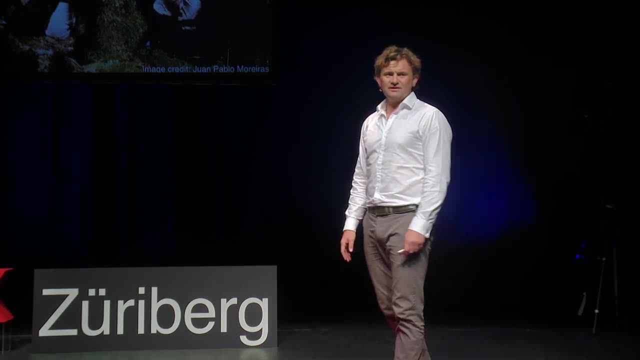 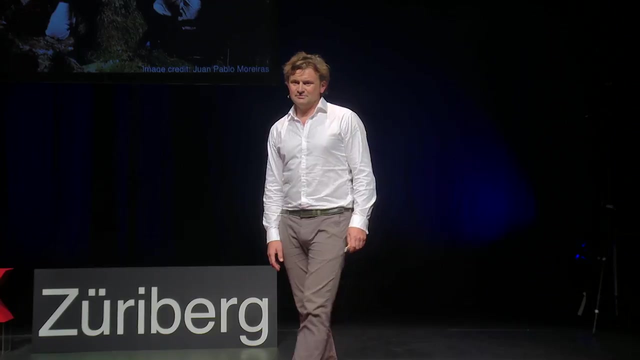 and rebel outfits, remnants of Congo's civil war Hiding out. there are also poaching and criminal gangs, and it's probably the most dangerous place in the world for a tiger. We also need to do some conservation. Wednesday night, Watch and review this series of 12 shows. 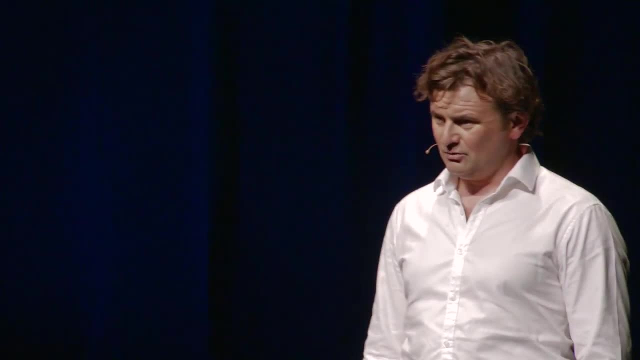 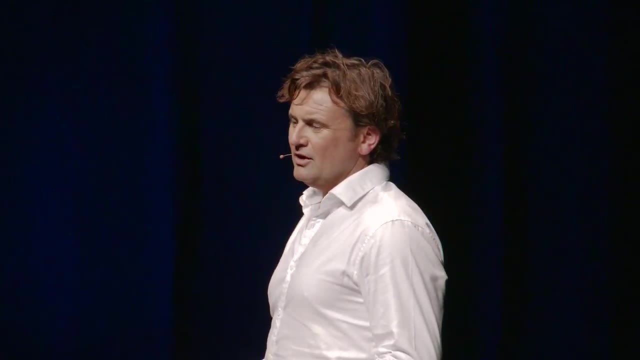 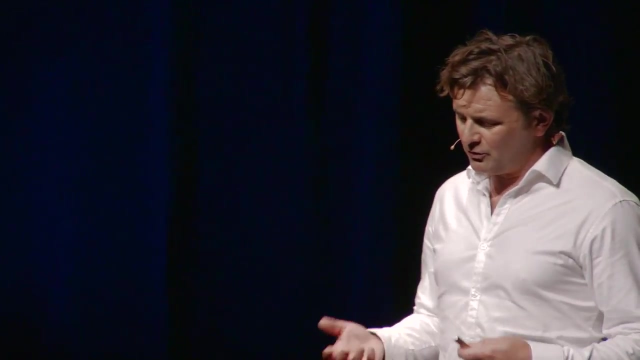 by Miles meters. uranNowcom. Enjoy. Choose your answers to today's questions Q&A P related And we'd like to wish you peace, Bye, See you next week, Bye, Bye. potential to cause enormous damage, such as here in Cambodia, where forests are being 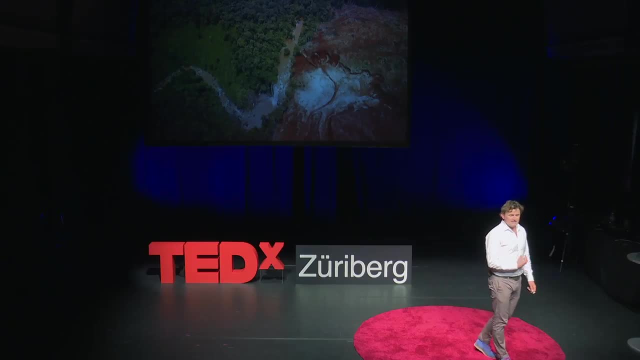 wiped out and the riverways are being polluted. What we need is people who understand these businesses. We need environmental impact assessment specialists, We need business specialists and strategists, We need lawyers And, fundamentally, we need people who understand these businesses and are prepared to work within them or with them. 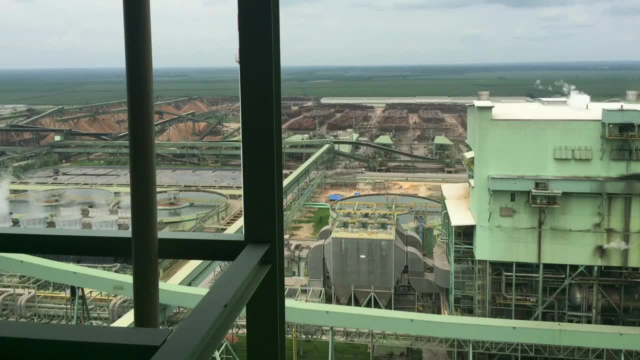 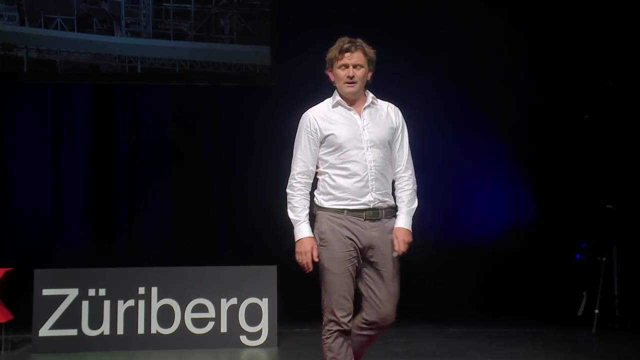 This is a paper and pulp manufacturing plant in Sumatra. It's owned and operated by a company called April, one of Asia's largest paper and pulp manufacturers, And they are responsible for decimating huge swathes of forest across Sumatra. But they've realized the error of. 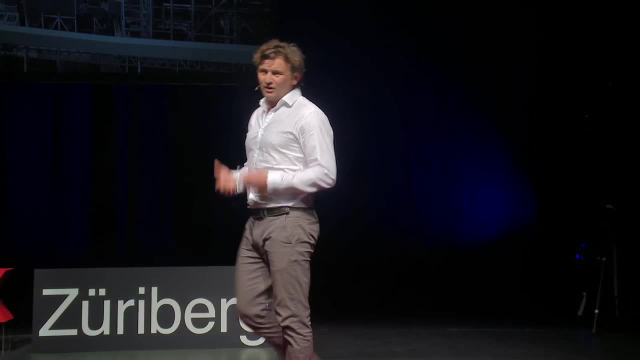 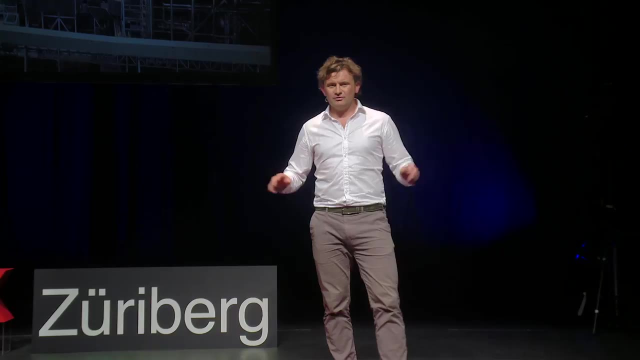 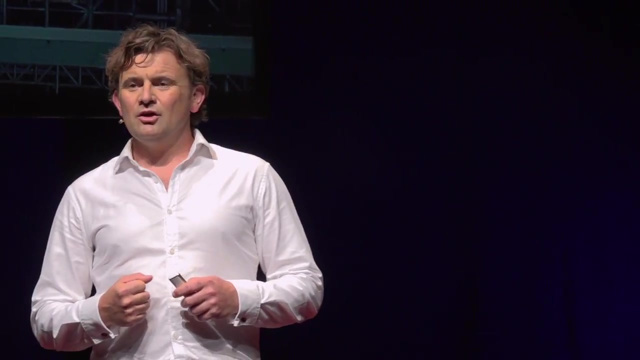 their ways and they're now solely reliant on plantation timber, And our role with them is to maximize the potential of the remaining forest and to use these plantations to make wildlife corridors, Crucial corridors that allow what wildlife is left to roam free, I suppose. in summary, 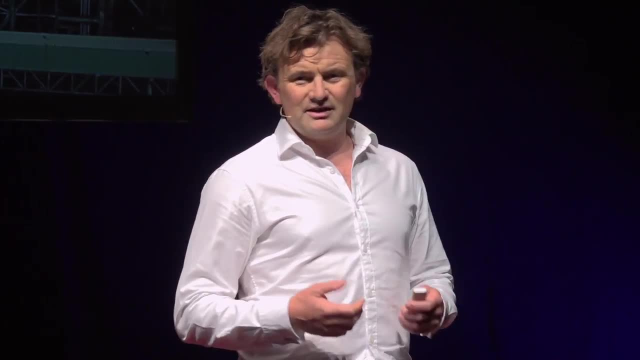 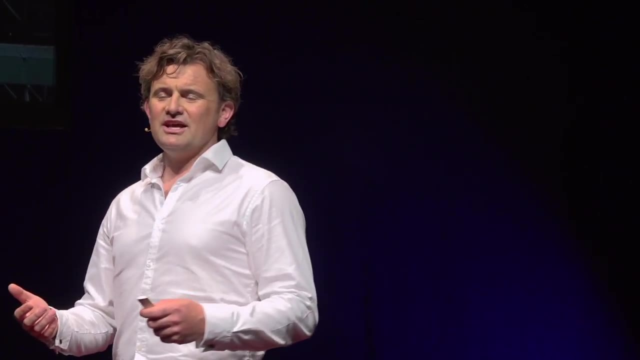 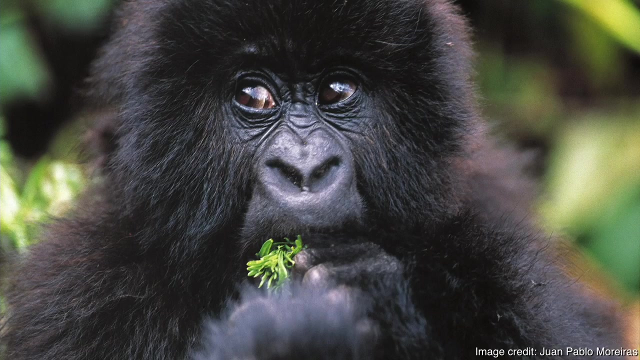 we've realized that to have impact, we have to engage with the people that have the potential to cause the most damage. So this is a lot of negative chat, And what I want to do now is share two stories of hope with you. The first is the International Gorilla Conservation Program Just over 30 years ago. 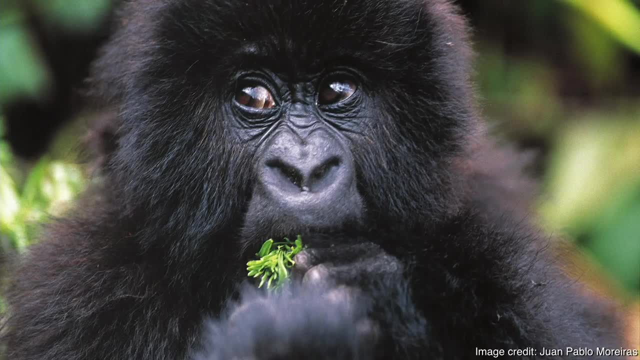 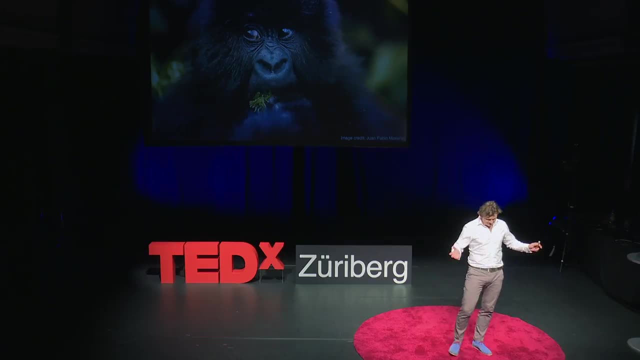 there was a lady called Diane Fossey who was living with the gorillas And she realized they were at a critical point. There were only about 300 left and their habitat was being wiped out. So who did she call David Attenborough? David came down and saw for himself. He shot film and 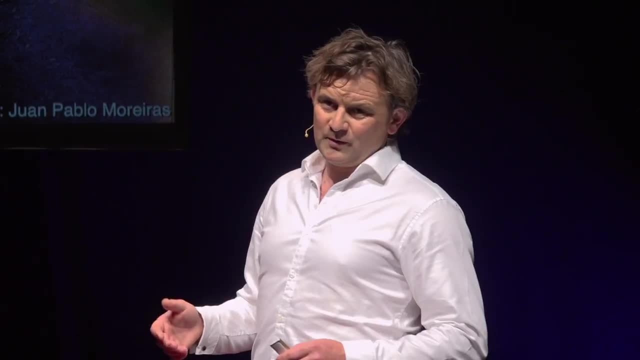 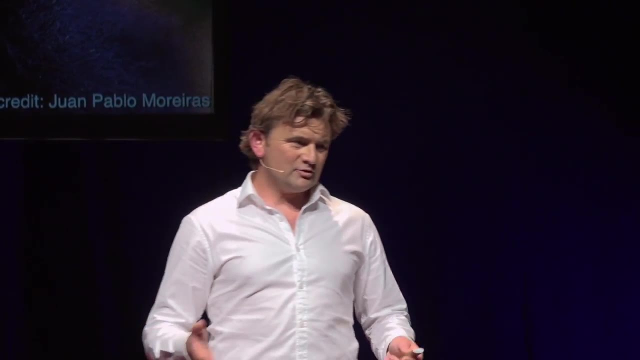 he went back to the UK And, to cut a long story short, the International Gorilla Conservation Program, IGCP, was formed. It's a collaboration between FFI and WWF, And the story goes a little like this: If you protect the forest, you protect the critical habitat that the 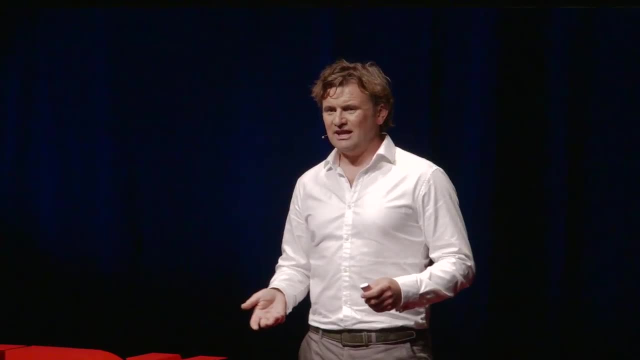 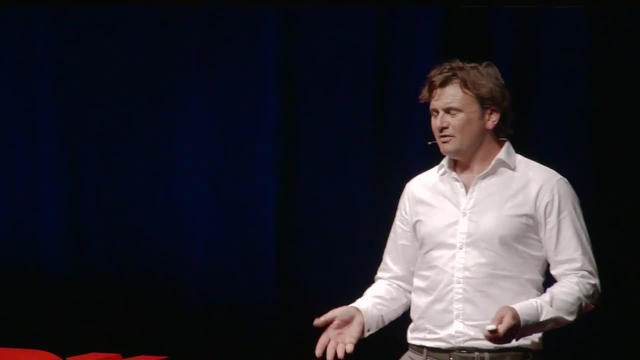 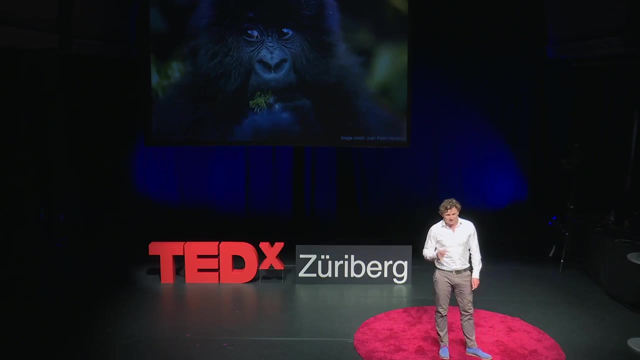 agriculture programs alongside ecotourism, This gorilla tourism, which is now worth in excess of 200 million US dollars a year and, amazingly, it's the single biggest contributor to Rwanda's GDP. Remember, it's a very small country, But the best news of all, there are. 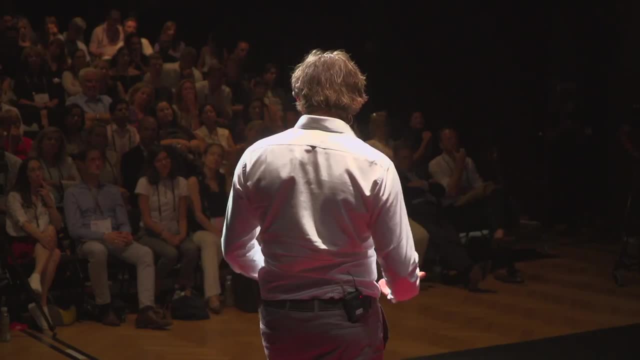 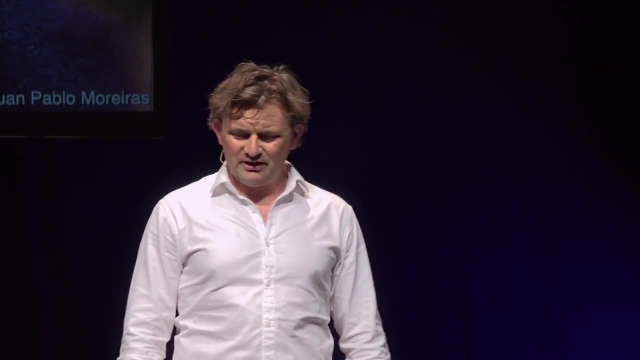 now over 1,000 mountain gorillas living there. And the other thing: it brings enormous pride to the local communities: employment and and the local communities, employment and employment in an area that's been through so many troubles in its recent history. 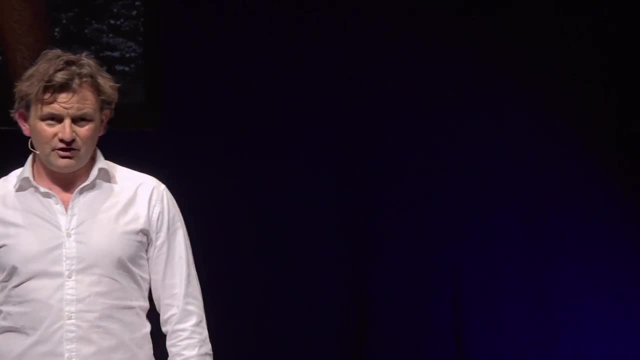 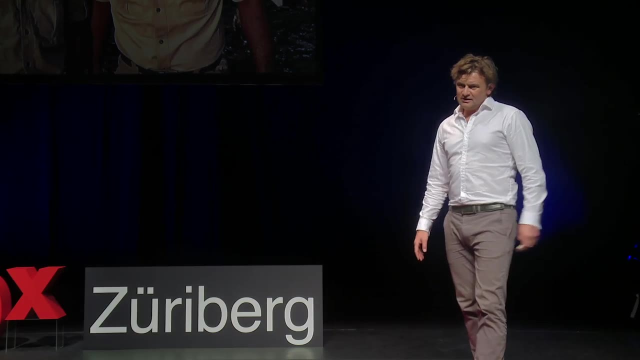 The second story's very different. It's about two twins I met six months ago Now. these are very intelligent and worldly guys, And what sets them apart is they come from enormous privilege. They've always been interested in nature, but they're not conservationists. They've 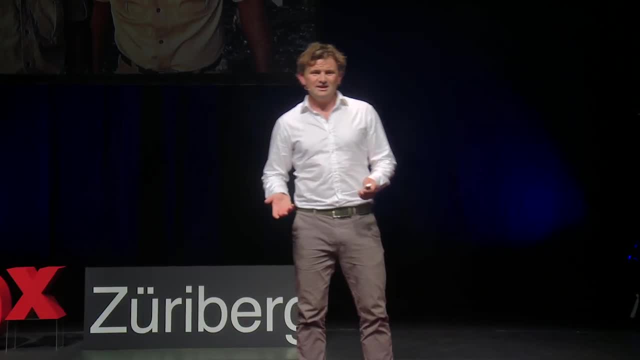 never really been to Africa, they've never experienced the savanna grasslands and they've never crossed an ocean. They certainly didn't keep pet worms and collect snail shells, But the thing is they love to enjoy nature, And the reason why they're here is because they're. 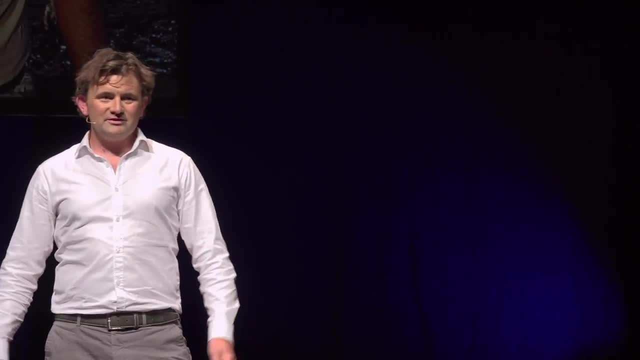 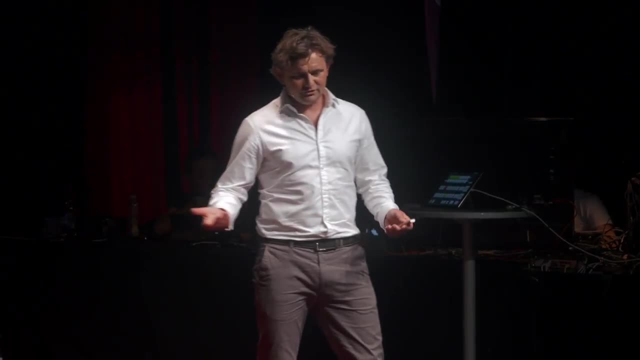 loved Sir David Attenborough and one day, as only people like this can do, they decided: you know what this guy makes sense. we're going to write to him and ask what he can do and again, to cut a long story short, Sir David introduced me to them and I took them to Africa to see our major projects. 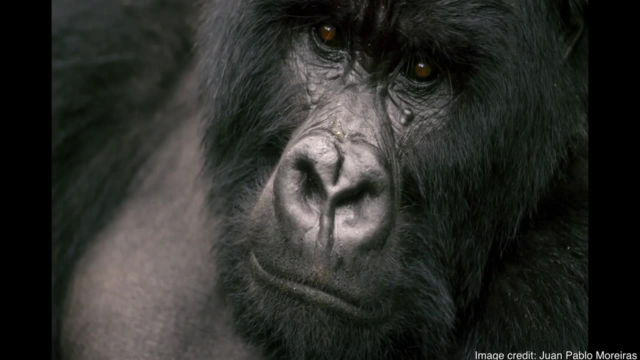 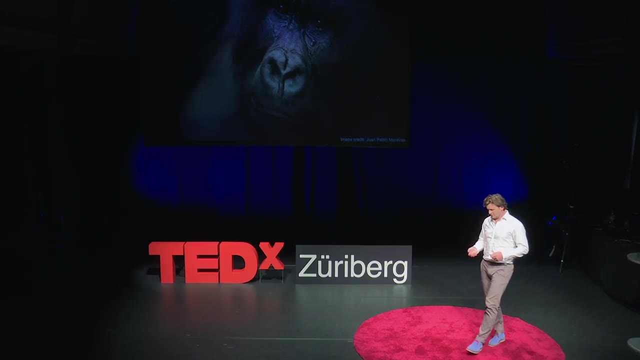 which included the iconic mountain gorillas. they've lifted the lid and Africa has got under their skin. they've seen, heard and felt what real nature is like and we now have two new lifelong conservationists who come with power, influence and significant resources that they're making 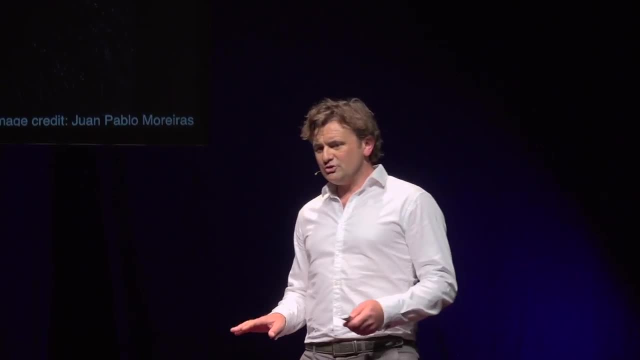 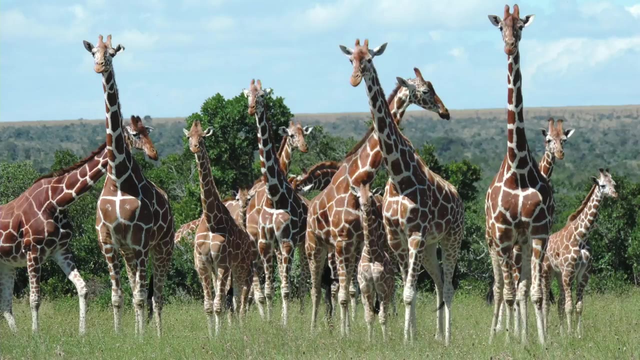 available to help us in this battle now. these are good news stories that I believe we should celebrate, and we should celebrate them together. this is a tower of giraffes, by the way, because collaboration is key to success. there are many examples within the NGO world, but I just want to. 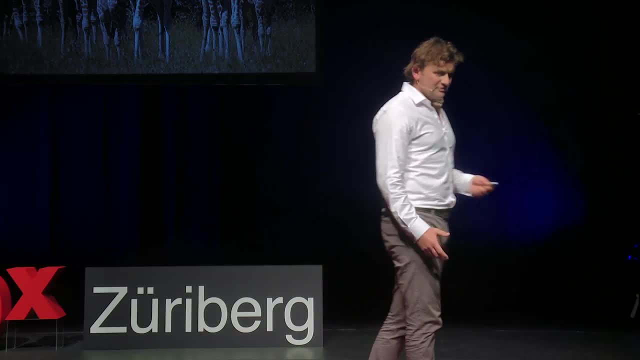 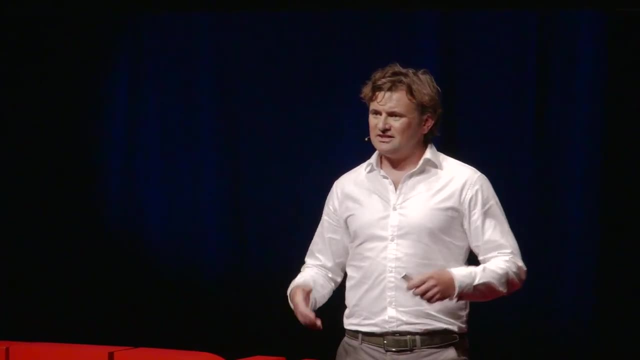 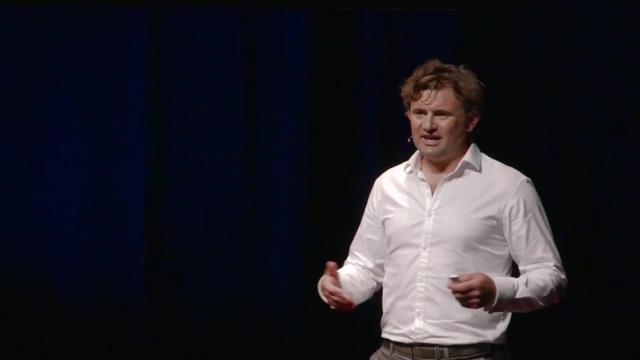 quickly pick up on something called wild labs. it's a community of conservationists, technologists, engineers, data scientists, change makers- and what they do is they get together and they share ideas, they share technological innovation tools and they're coming up with new solutions to age-old conservation problems. 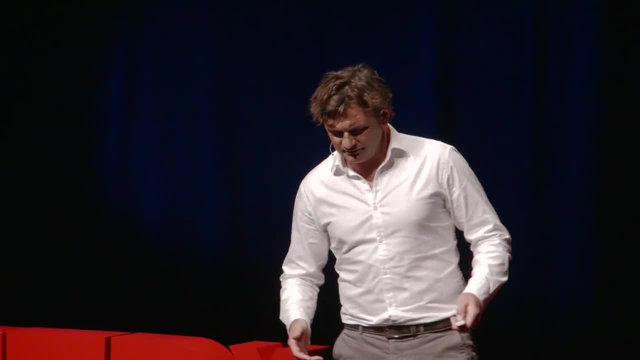 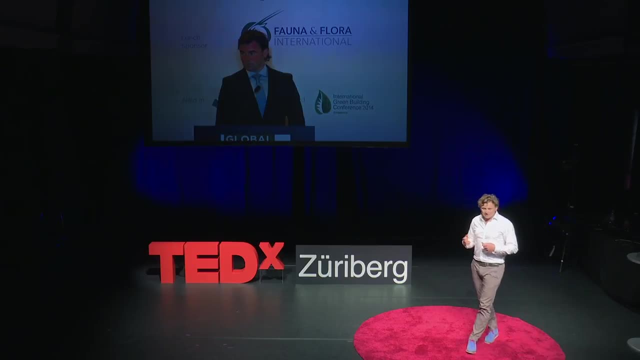 in short, the conservation world is recruiting for new skills. so who else do we need? well, we need people who in suits, who can talk a bit better than me, but but I really think that we need to maybe follow the lead of men like Shackleton we need